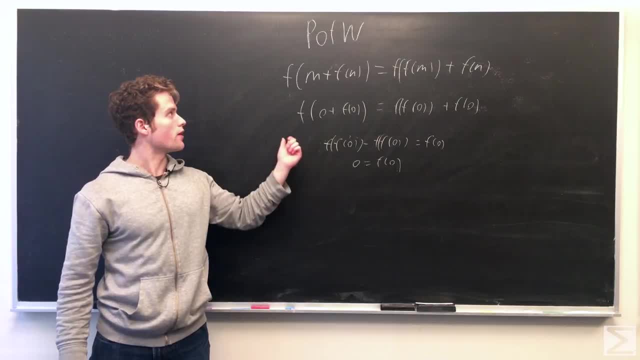 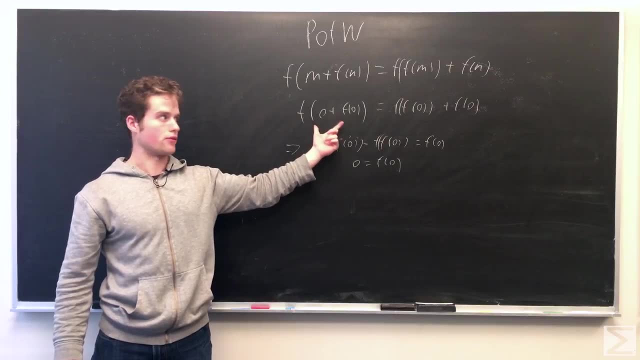 So the first thing we can do is just plug in zero everywhere. So f of zero equals zero Plus f of zero equals f of f of zero plus f of zero. The thing on the left is just f of f of zero. So we're going to subtract off two these two f of f of zeros. 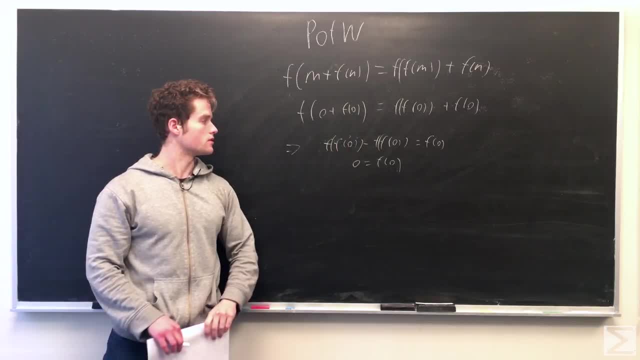 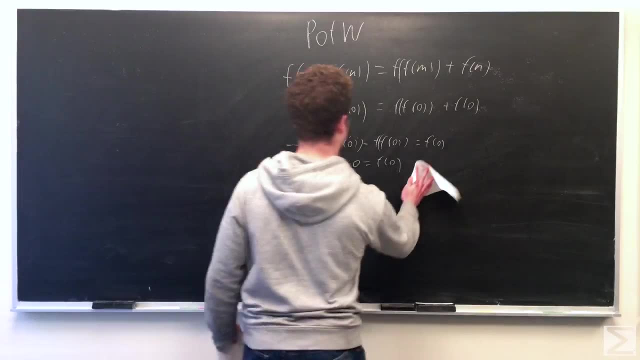 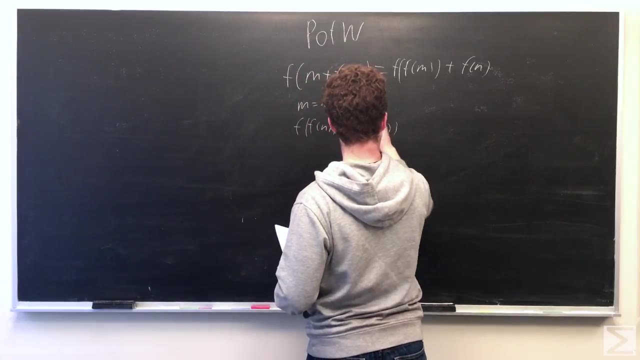 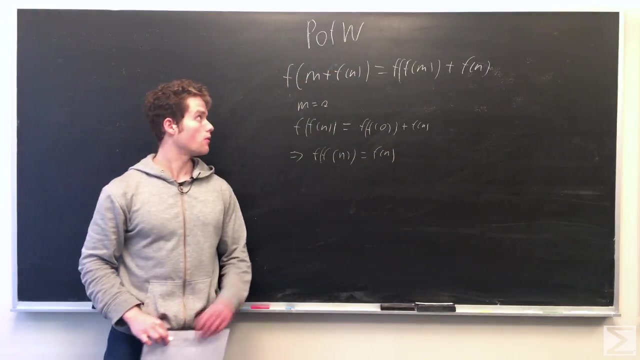 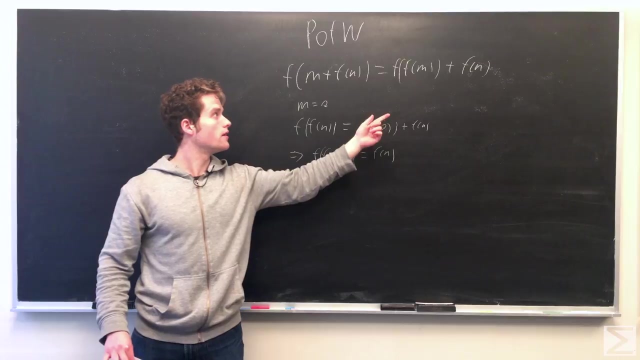 And we're left with zero equals f of zero, which is simple enough. So the next thing we can do is just plug in f of f of n. So we just plug in m equals zero. This becomes f of f of n. f of f of zero is just f of zero, which is zero. 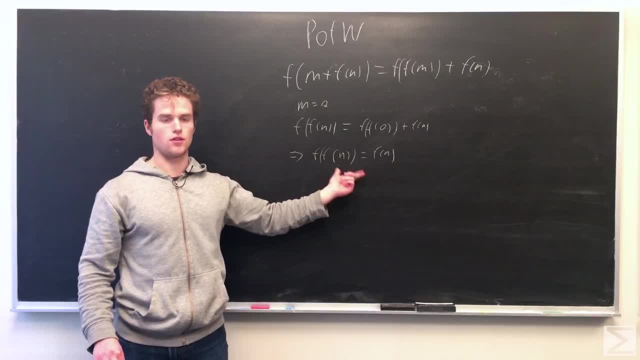 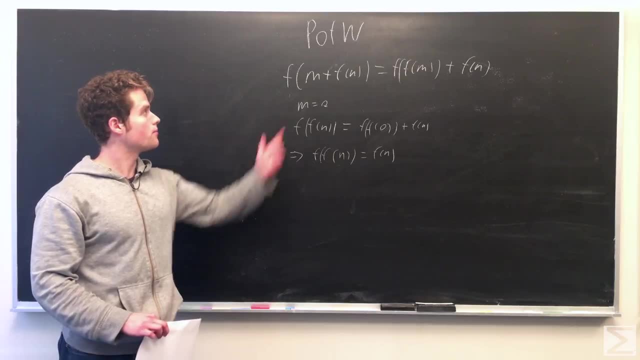 And then f of n stays f of n And we're left with f of f of n equals f of n. So this is another tidbit of information. Now, another thing we can do: we can plug in for m. here We're going to substitute m plus f of n. 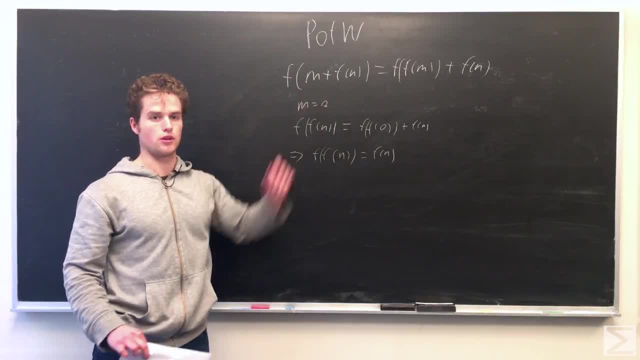 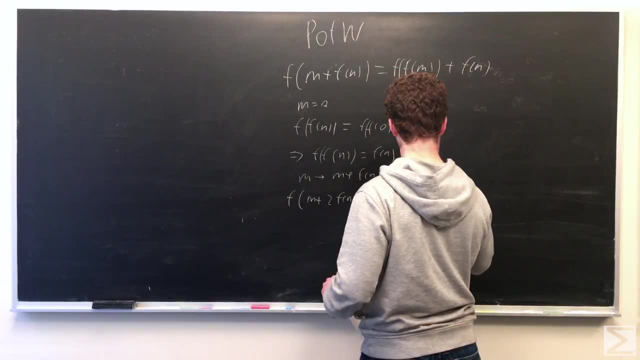 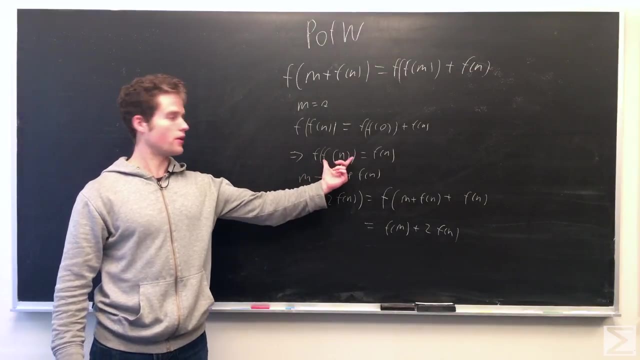 So we're going to try to plug in f of f of n. We're going to try to find out what m plus two f of n will give us. So note, because we know f of f of n equals f of n, that f of f of m here we can just write that as f of m. 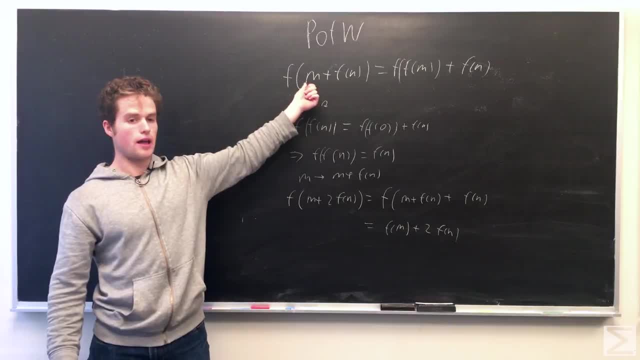 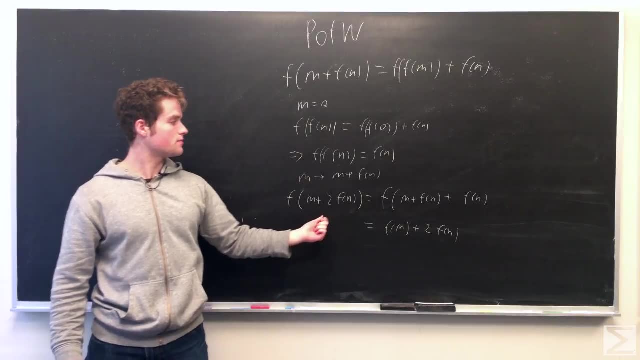 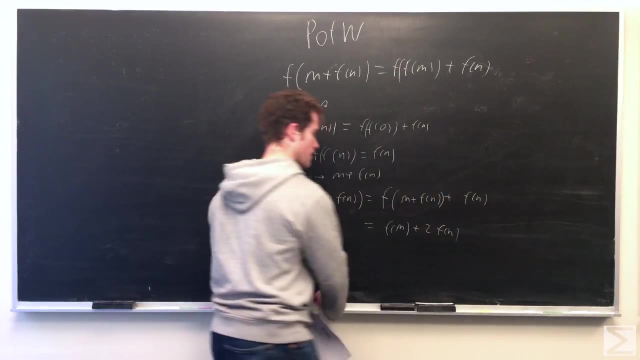 This simplifies this equation a little bit, So substituting m plus f of n for m, here we're extending m to m plus f of n, So f of m plus two f of n equals f of m plus f of n, f of m plus f of n plus f of n. 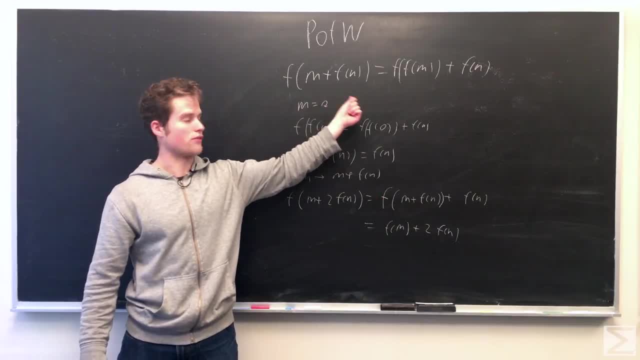 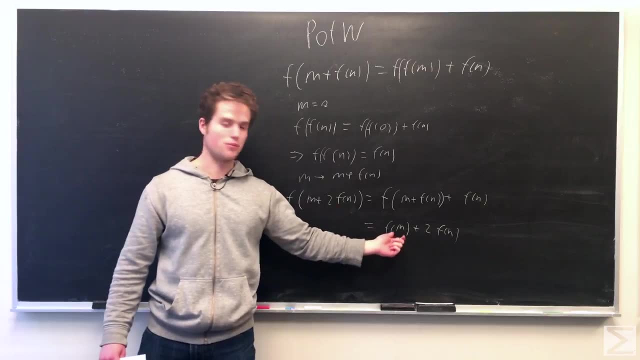 f of m plus f of n from our original functional equation is just f of m plus f of n. So this is equal to f of m plus two f of n. So f of m plus two f of n equals f of m plus two f of n. 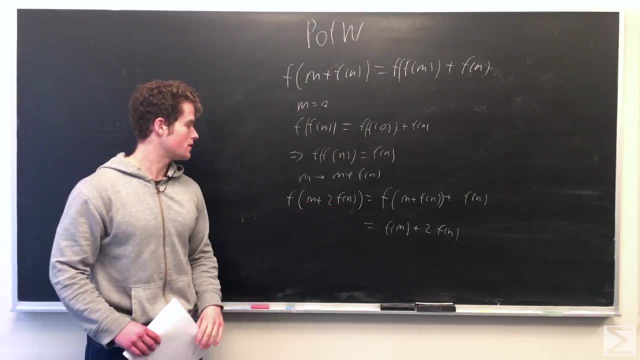 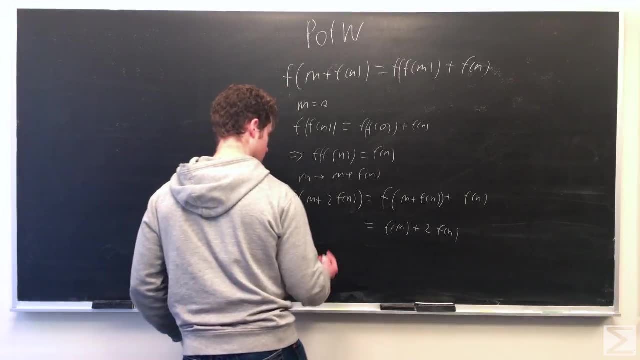 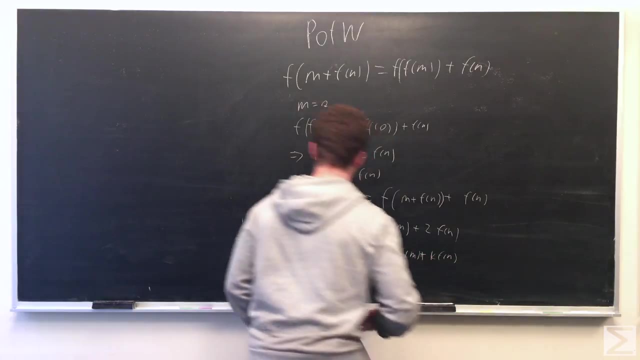 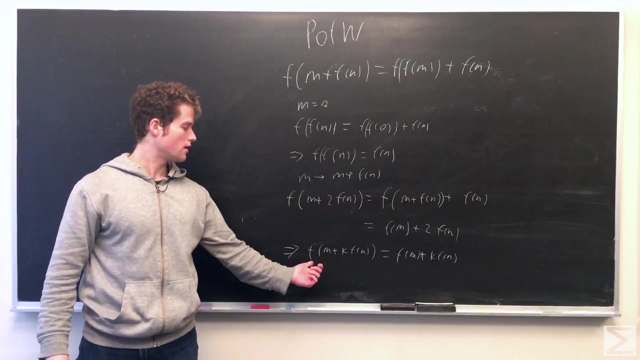 So we can kind of. it's a little bit linear, Yeah. so we can do this repeatedly and we'll get, If we keep plugging in m plus f of n for m here, this will become m plus three n, m plus four n, et cetera. 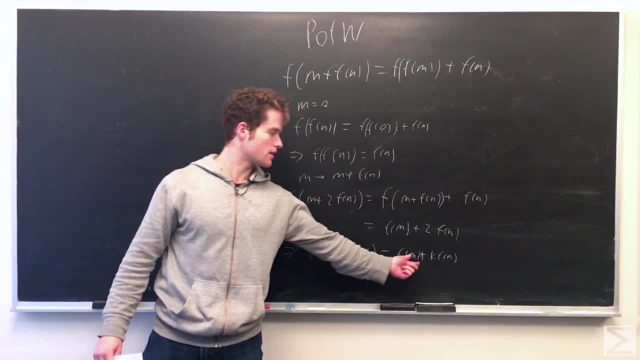 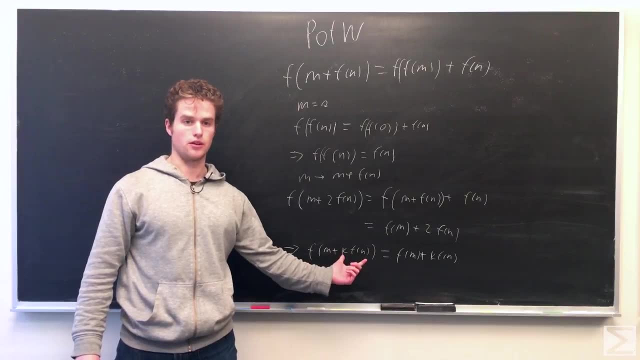 So in general, m plus k f of n equals f of m plus k f of n, where k is some non-negative integer. And so this is another little bit. So that's a little bit of information. Now we can do one more, another thing. 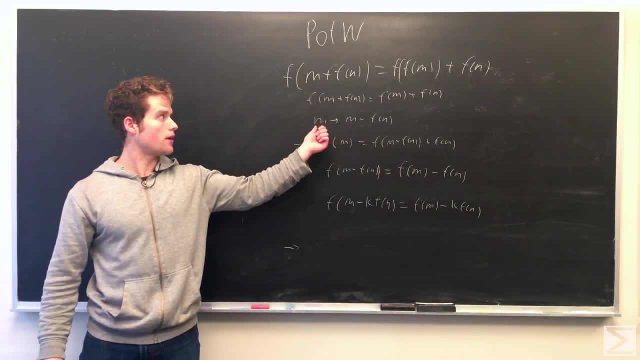 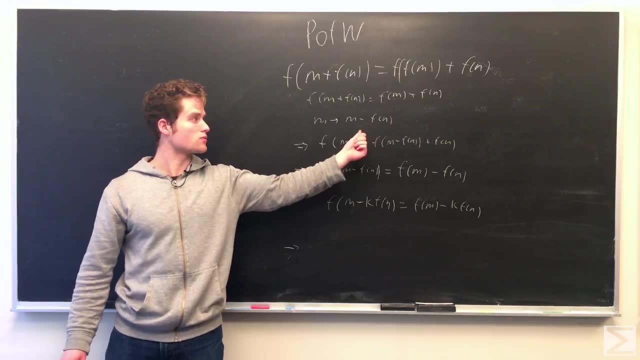 Another thing we can do: we can plug in m minus f of n. we can plug in m here, being careful that this m minus f of n is greater than or equal to zero, because we still want to be in the non-negative integer, which is where this is defined. 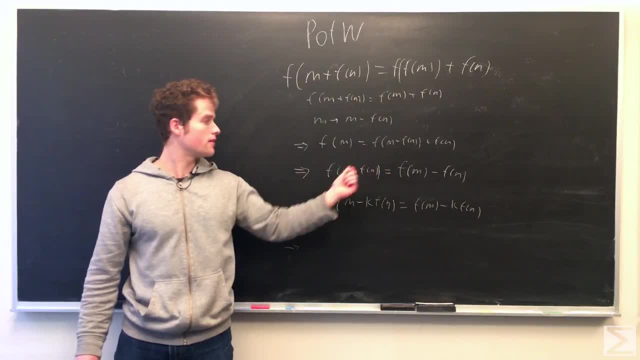 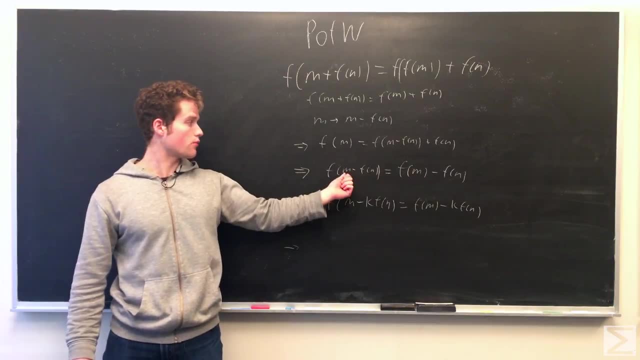 So doing that we get f of m equals f of m, minus f of n, plus f of n. We subtract off f of n from both sides. We get m minus f of n equals f of m minus f of n. And notice, if we keep repeating the substitution saying m to m minus f of n, 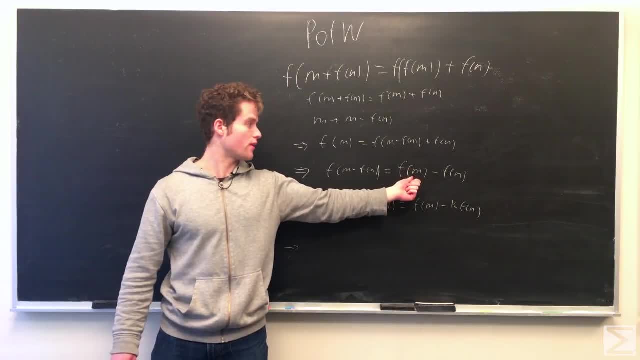 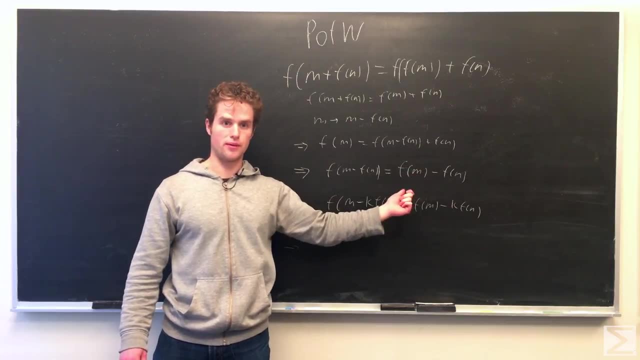 this becomes m minus two f of n. m here is f of m minus f of n, Which is- we can use this to get: that's equal to f of m minus f of n, minus f of n, or f of m minus two f of n. 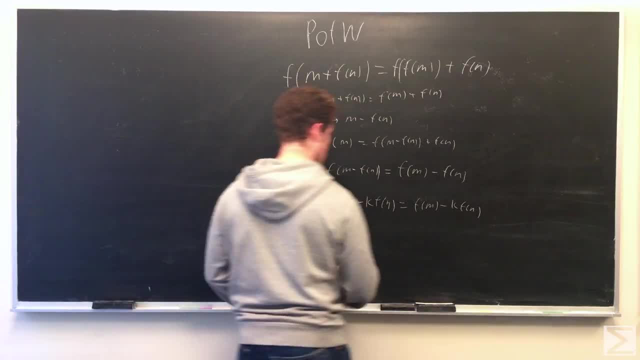 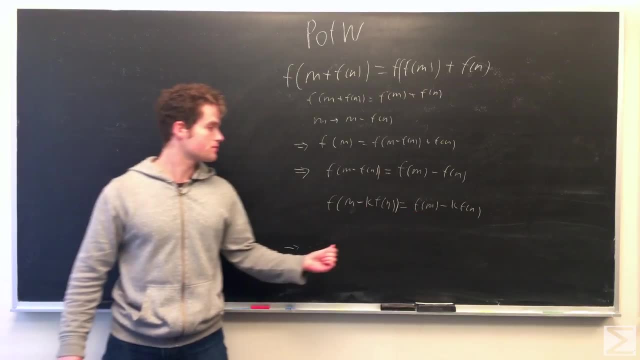 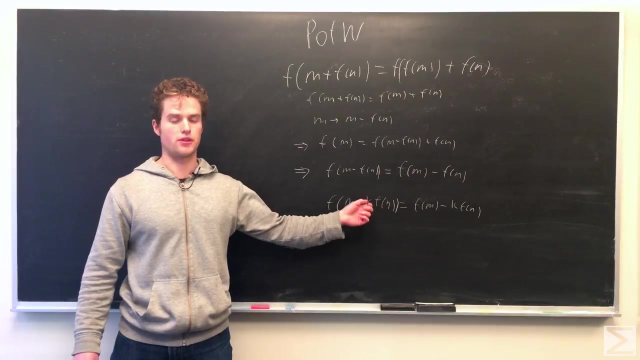 And we repeat this: to get in general, f of m minus k f of n equals f of m minus k f of n, And so this. so now, so we know now, k can in fact be positive or negative integers. from what we learned previously. 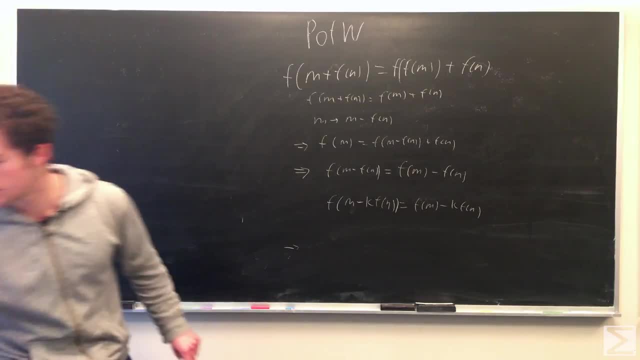 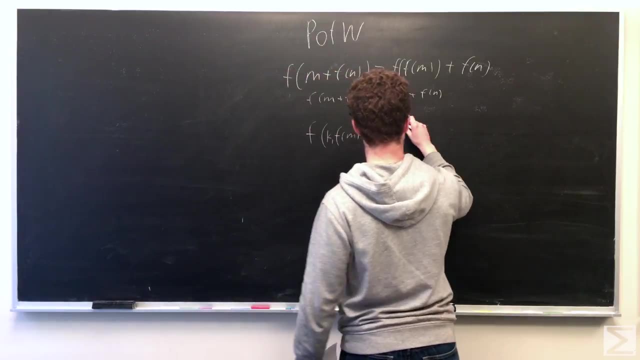 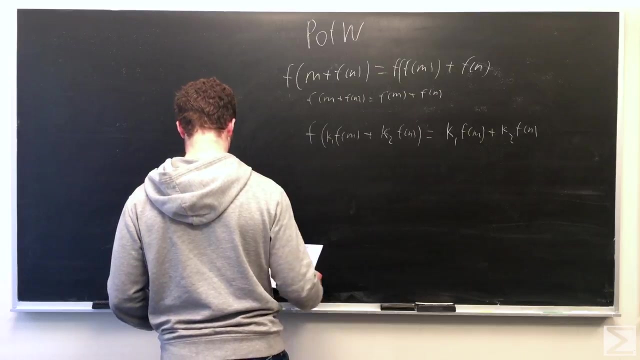 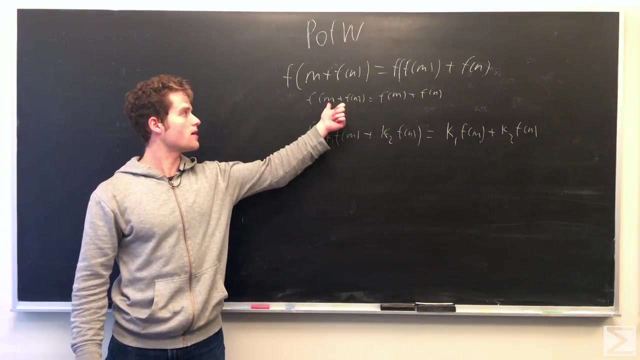 So from these two bits we can do another thing. So because so with our equation here instead of m we can write f of m. It doesn't change anything, because f of f of m is just f of m. 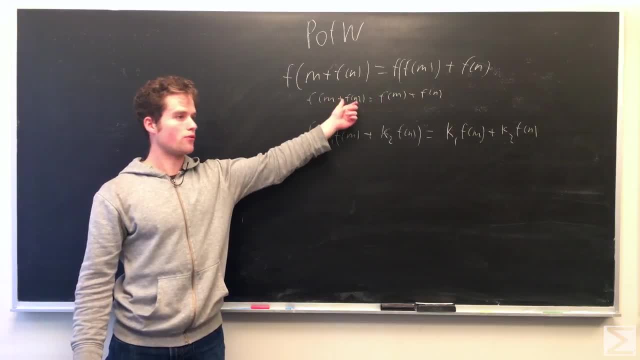 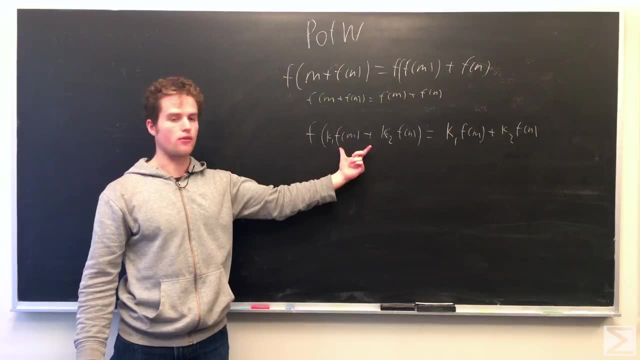 And then we recall we can, for f of m, f of n, we can repeatedly add this to track f of n's, f of m's to this, to get a form k one f of m plus k two f of n. 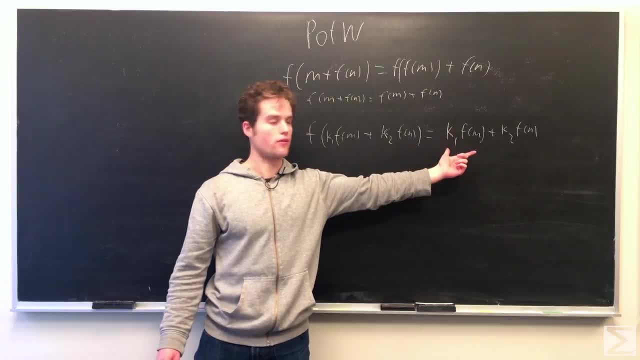 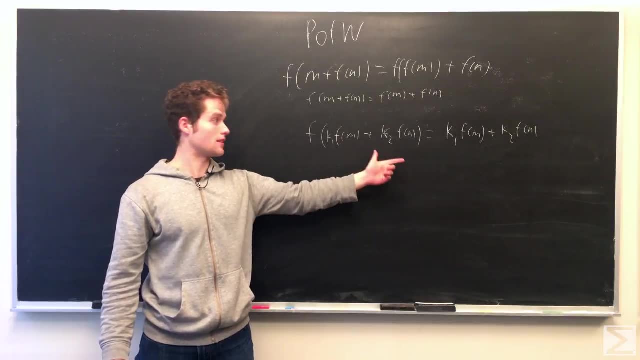 And this will be equal to the same thing: k one f of m plus k two f of n, Where k one and k two are just integers. and from what we previously learned, these can be integers and this will stay a fixed point of our function. 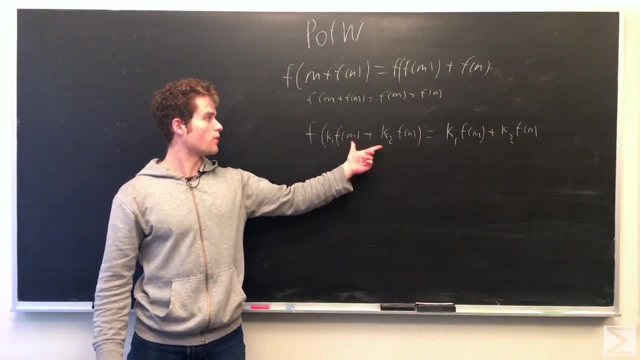 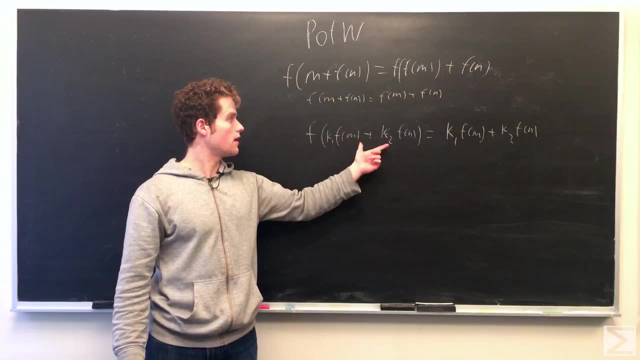 And so it's a common known fact that so we take any two uh integers in the range non-negative integers in the range of f, And so we can get that their greatest common divisor is in fact a fixed point of f. 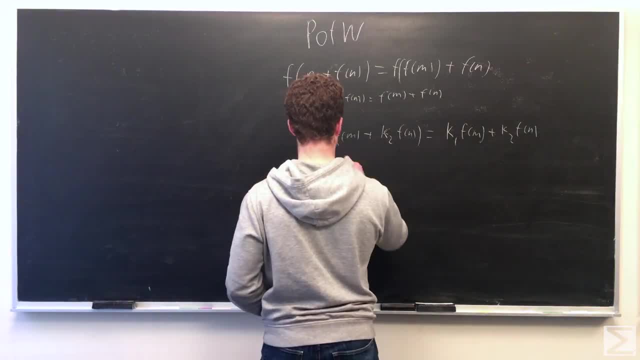 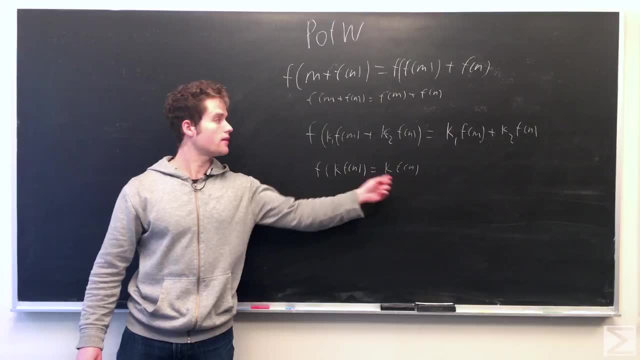 And also note that, note just saying, one of these k's equals zero. we have f of k. times f of n equals k f of n And here, because we can do this, we can say: really the range, there is some integer d that. 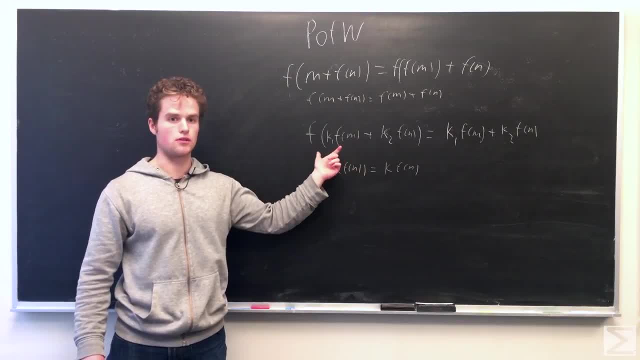 divides every number, every integer. So we can say, really, the range, there is some integer d that divides every number, every integer in the range of this function. Because if there wasn't, if there was some integer that did not divide d, we can do this. 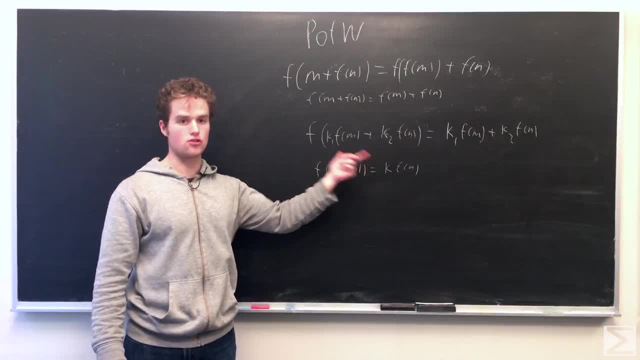 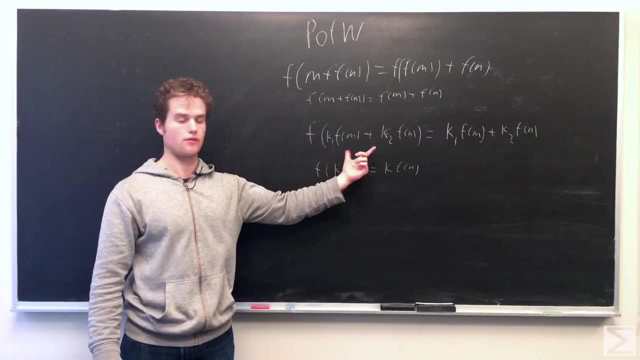 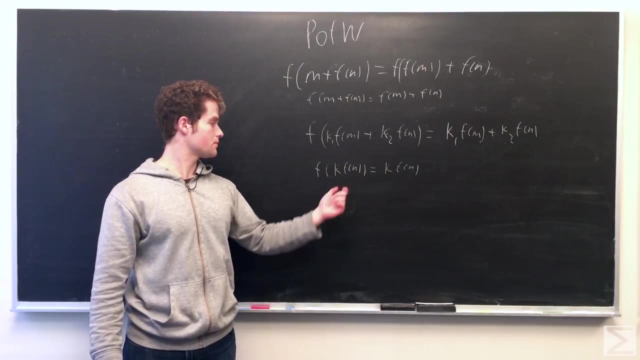 we can find out what their greatest common divisor is, and then that integer would be something that divides every number in the range of f. So we have some number d that divides every number And we also note that. so if f of n is equal to this d, because d is clearly going to be in our range- 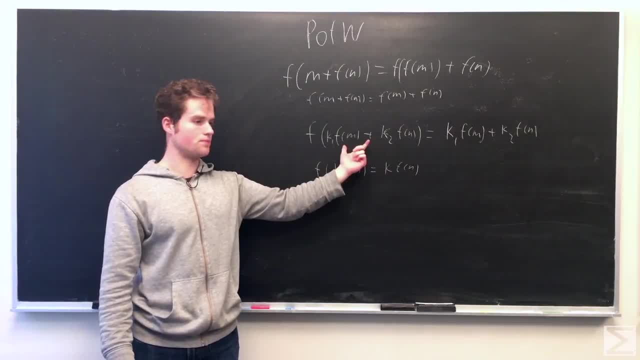 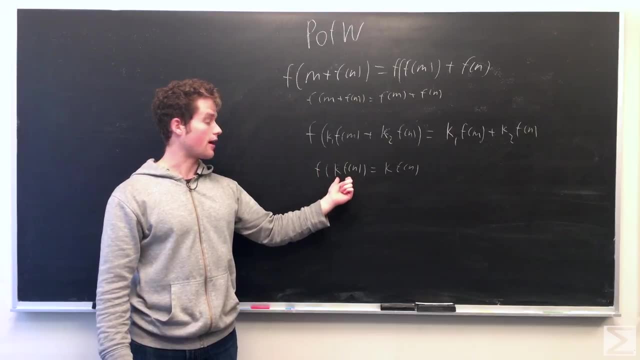 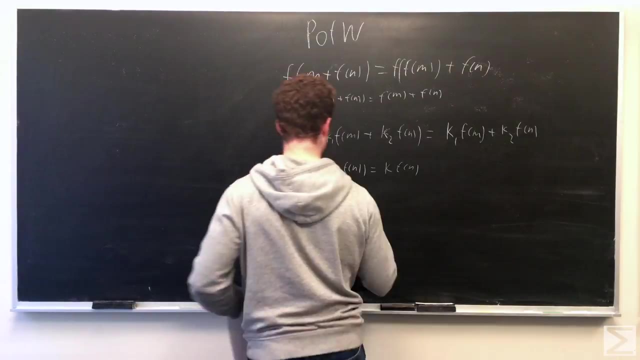 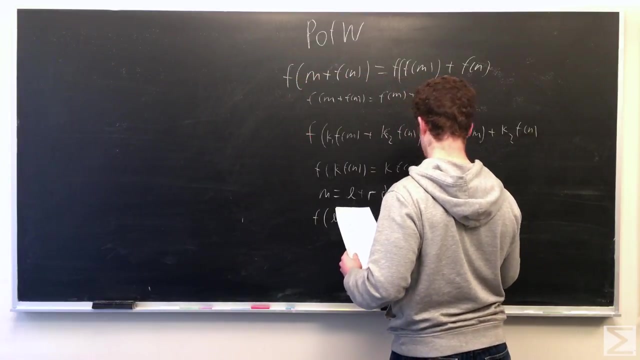 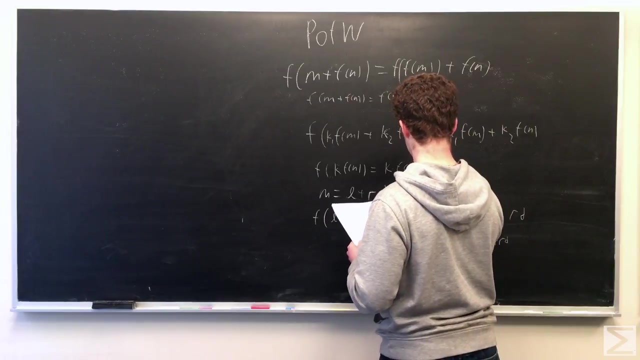 any multiple of d is a fixed point, And because every point in our range is divisible by d, our range is really just multiples of d, just some integer d, And so now we're almost done. So now we pick some nonnegative integer d. 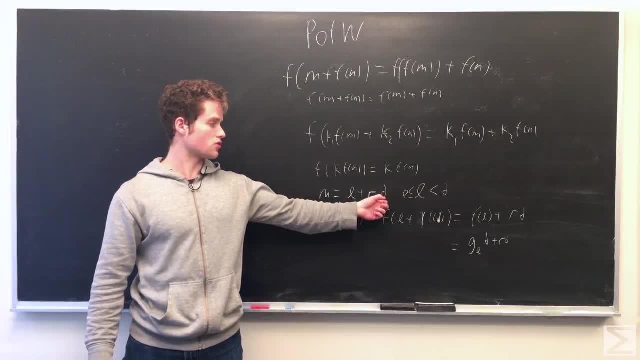 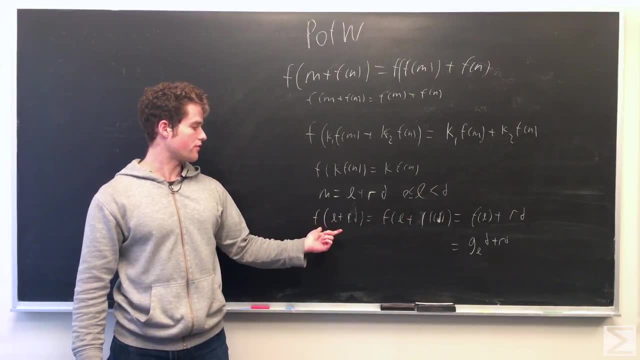 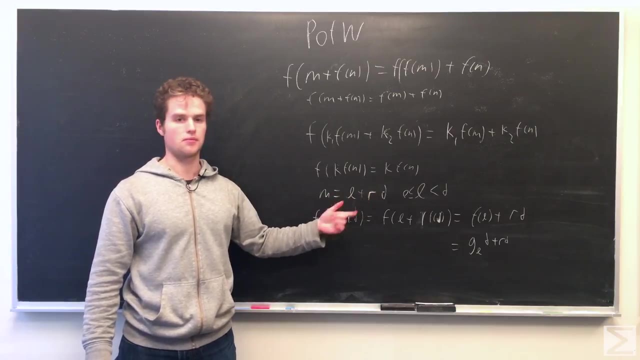 Yeah, We pick some positive integer d And we consider all l l greater than or equal to 0,. less than d, And we know f of l, we can write any integer as l plus rd where l is less than d by division algorithm. 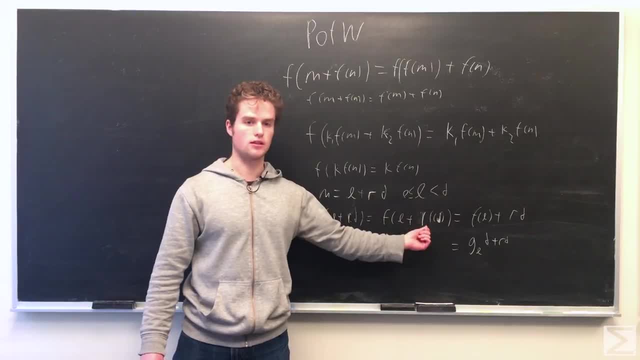 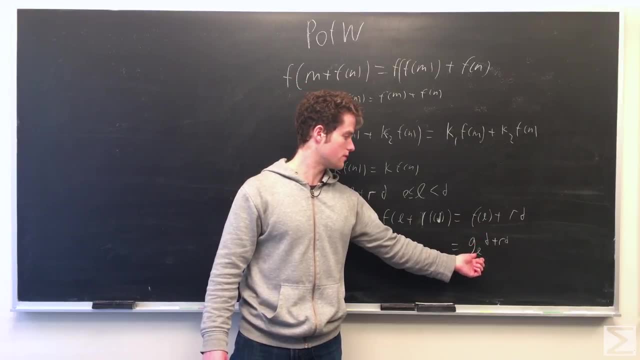 So f of l plus r d is f of l plus r, f of d, because d is a fixed point and this is just f of l plus r d, And f of l must be divisible by d, so f of l is just some g of l d plus r d.